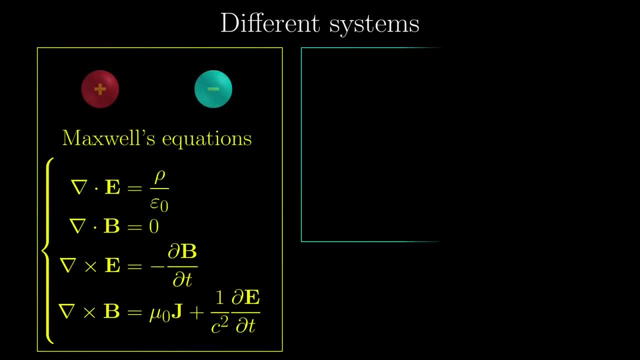 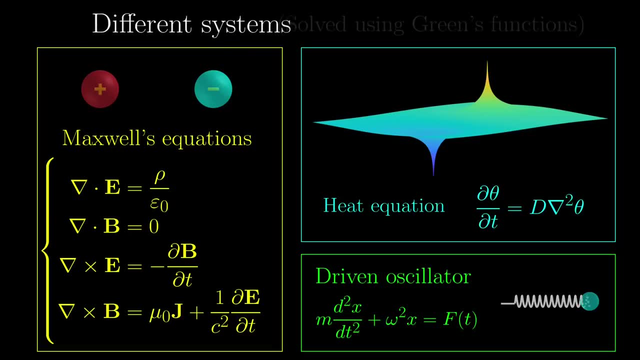 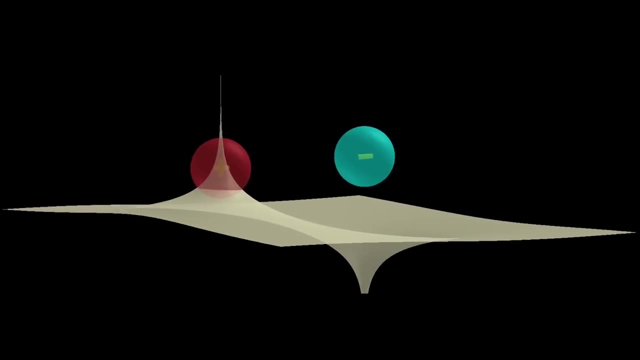 Lots of systems are governed by differential equations, which is why we want to solve them systematically. Green's function is a very powerful and clever technique to solve lots of them. To illustrate intuitively how it works, we will consider electrostatics, one of the problems. 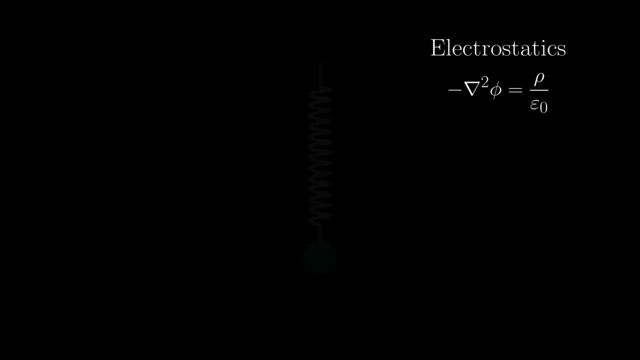 Green was interested in, and Newtonian mechanics, specifically an oscillator under some variable force. What is the common thing in these two equations? Well, they can be written in a very general form: Ly of x equals f of x. L is what's called a linear differential operator, which I 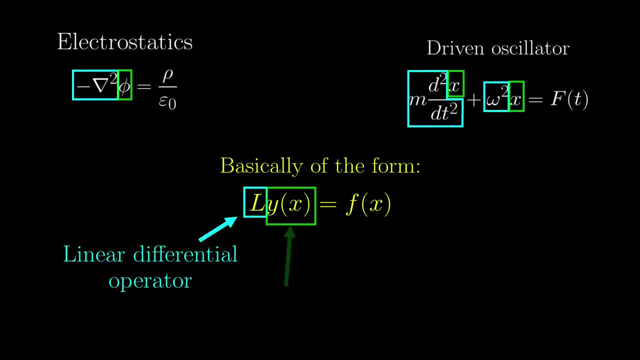 swear is not as scary as it sounds. y is a function of x to be solved and the right hand side is some other function, which we call the forcing term, which is given. Green's functions can deal with any equation like this. 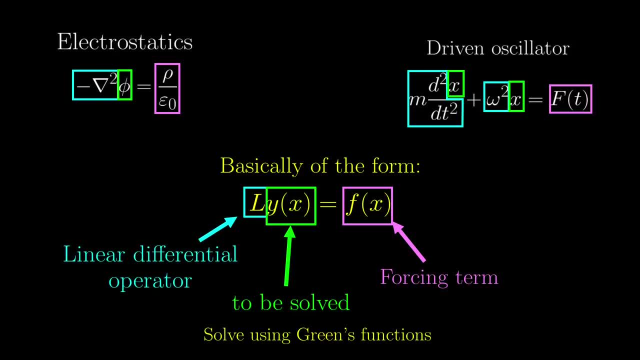 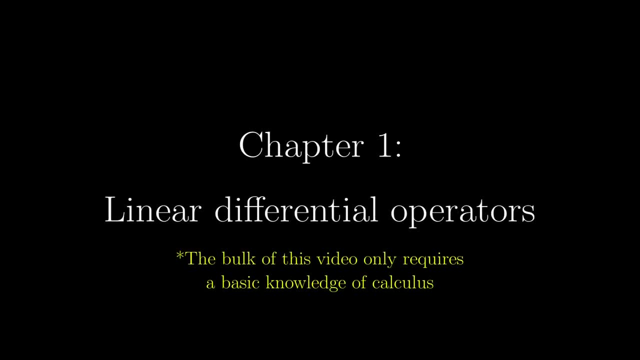 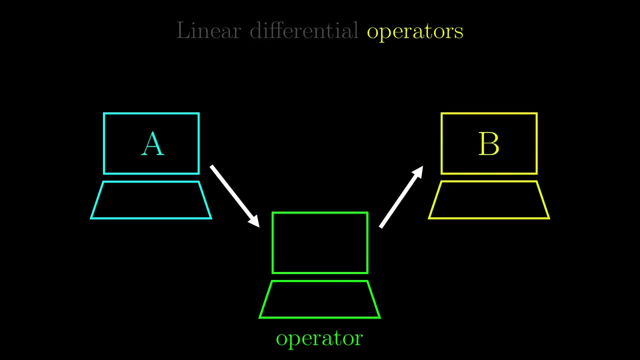 But first we have to talk about what linear differential operators are. We are going to explain each word separately. Operators in this context means a function that has a function a as input and the output being another function b. For instance, differentiation is an operator because the squaring function 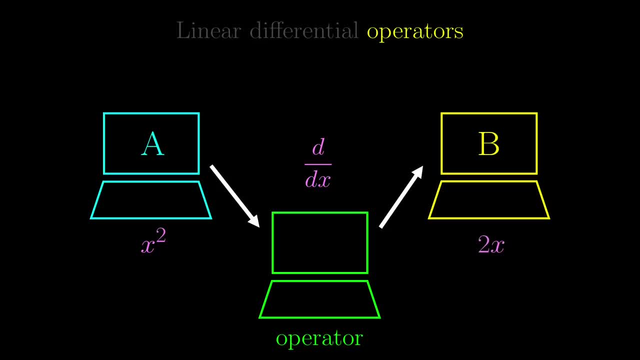 is made up of a function a and a function b, and a function b It's mapped to the doubling function under differentiation. So when we see an equation like this, it means that the function y of x, when fed into the operator L, becomes f of x. By solving a differential equation we mean recovering y of x. 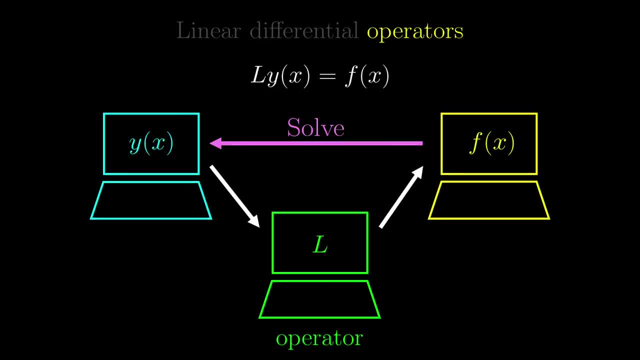 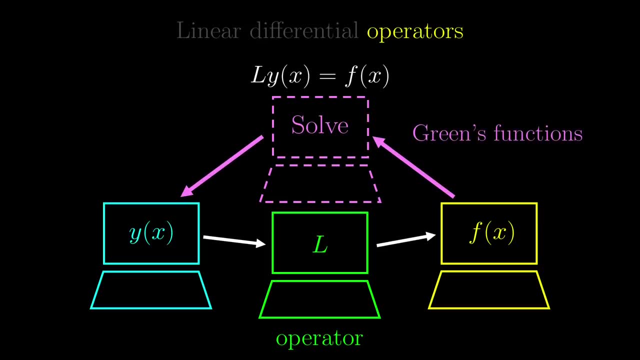 from f of x. So what Green's functions try to do is to sort of construct another operator that when the forcing term is fed, it outputs a function a and a function b and a function b. It outputs the desired solution y of x. So this explains operator. 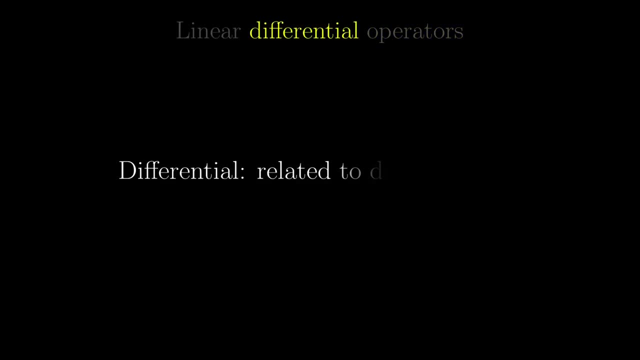 Differential doesn't have too much meaning. It simply refers to relating to differentiation. But here comes linear, Algebraically, this is the definition of linearity in this context. Essentially, the left-hand side says that we first consider a linear combination of two functions. 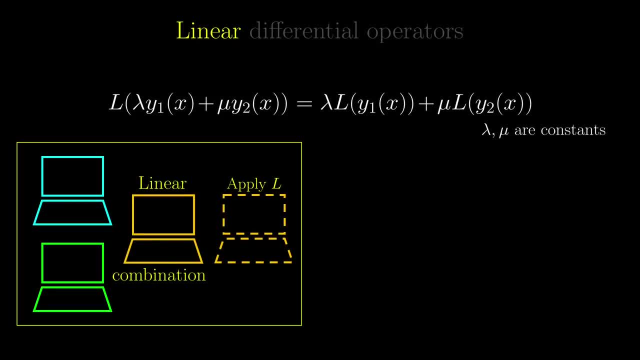 and then apply the opposite. This is the definition of linearity in this context. Essentially, the left-hand side says that we first consider a linear combination of two functions and then apply the opposite. The right-hand side thus thinks in the reverse order, by applying the operator to both functions. 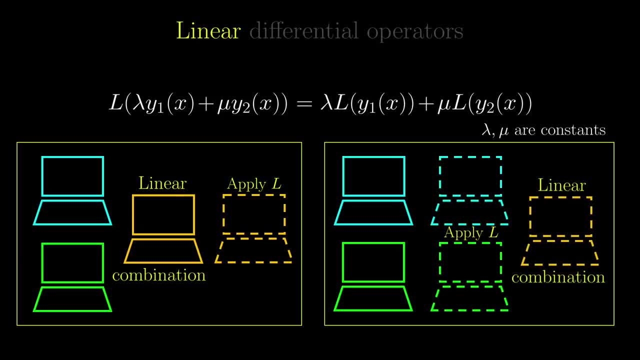 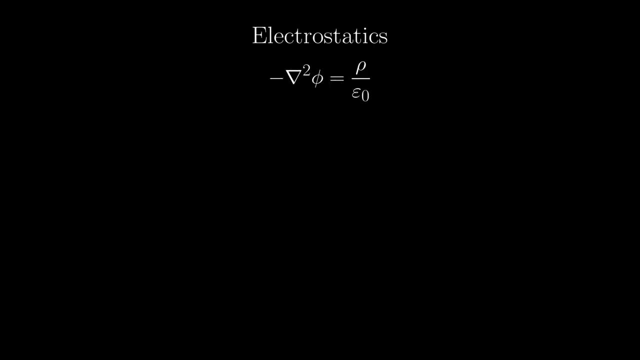 first, then consider the linear combination. The operator being linear simply means that the order of these two steps doesn't matter. But intuitively, what does this mean? Let's take a closer look at this specific equation for electrostatics For this video. 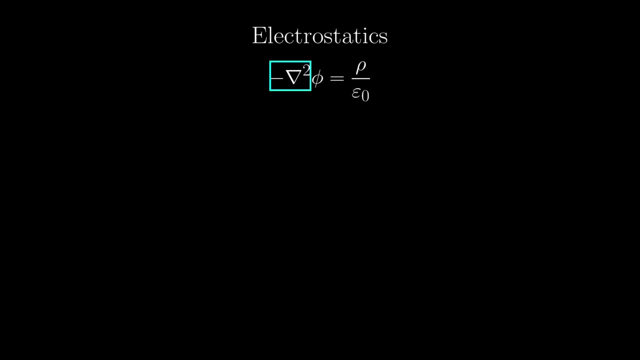 you don't need to know what this inverted triangle thing is, just that it is a linear differential operator. Phi is actually the electricity potential, which is a function of position. Rho is the charge density distribution, which again depends on position. Epsilon-0 is simply a. 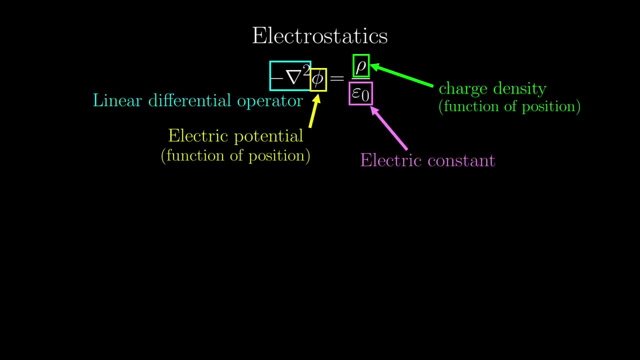 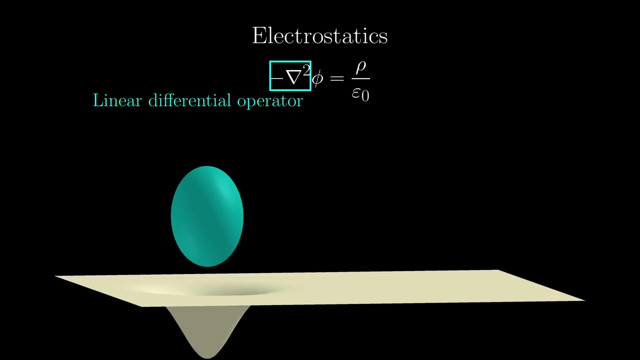 constant. Essentially, if you have a charged object with some charge density distribution, rho with charge density tension for al getan to equal 0 can generate an electric potential. an object with different charge distribution would yield a different potential, as dictated by the equation. If the two objects are brought together, you simply add up the potential generated. 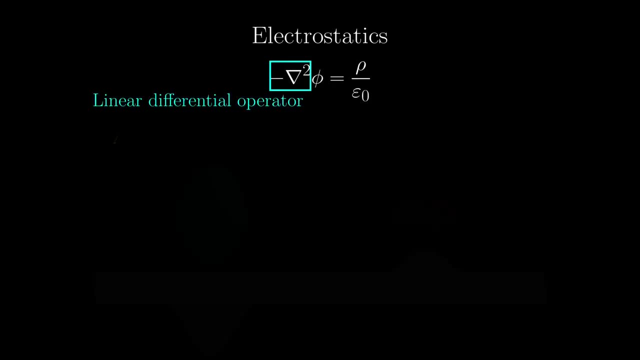 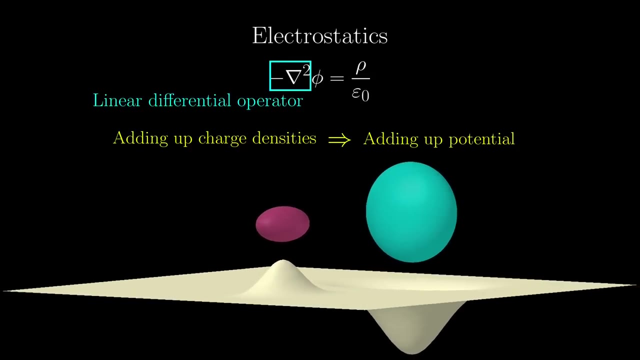 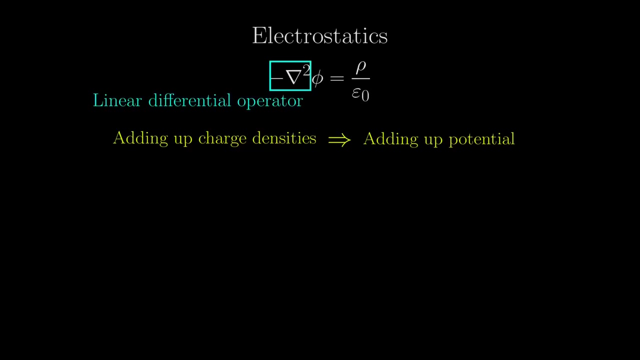 by each object. The fact that we simply have to add up the potential when putting two charge densities together defines linearity And, as we will see, Green's functions exploit linearity to the fullest. Let's return to the electrostatics example. More specifically, we want to take a 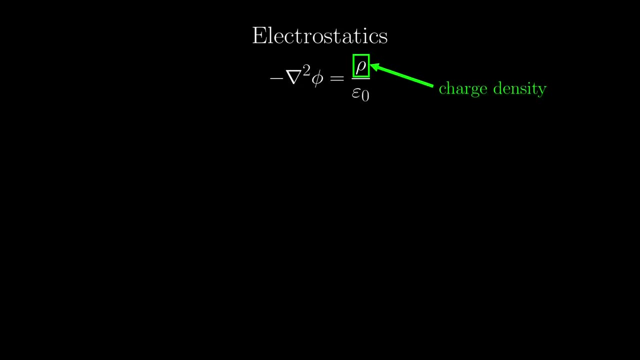 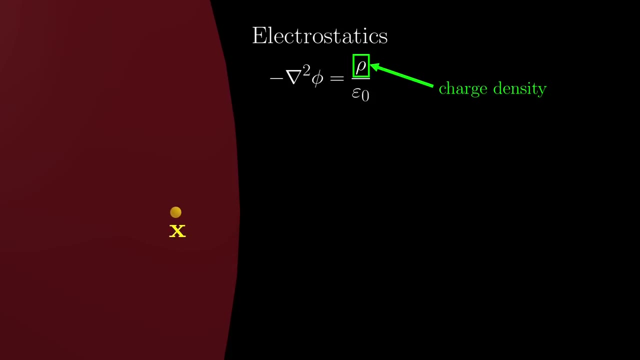 look at the charge density distribution From a practical point of view. how do we determine the charge density at position x? Well, the charge density is charge over volume in an infinitesimal region. Let's consider this relatively small region first, For the numerator, what is the charge within the region D? Well, it could be found by integrating: 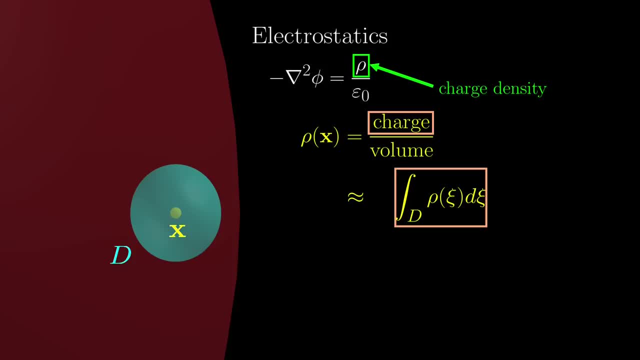 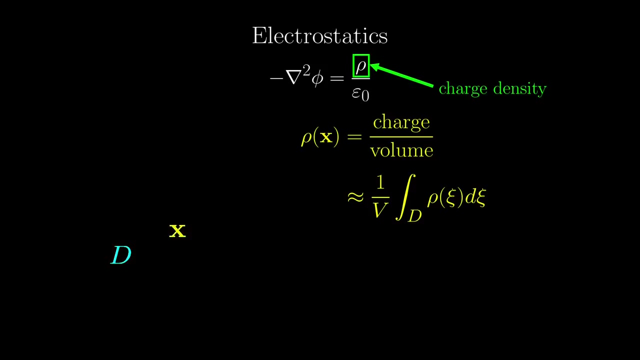 the charge density over the entire region, and I just denote V as the volume of region D. However, integrating over D is not ideal because the region is going to change in the limiting process. Instead, we use a trick: We integrate throughout the entire. 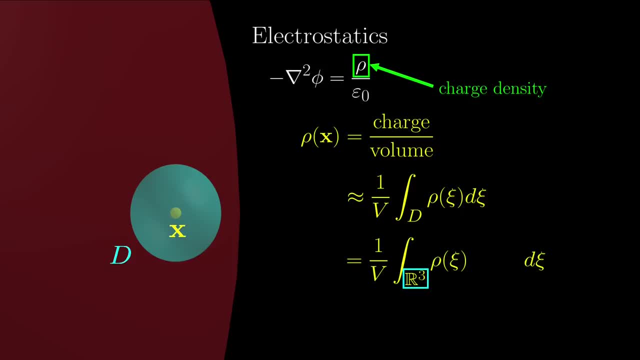 system. We integrate throughout the entire system. We integrate throughout the entire system. We integrate throughout the entire space. but we make a small change to the integrand We multiply by a simple function denoted by 1, with a subscript d. This is called an indicator function in this. 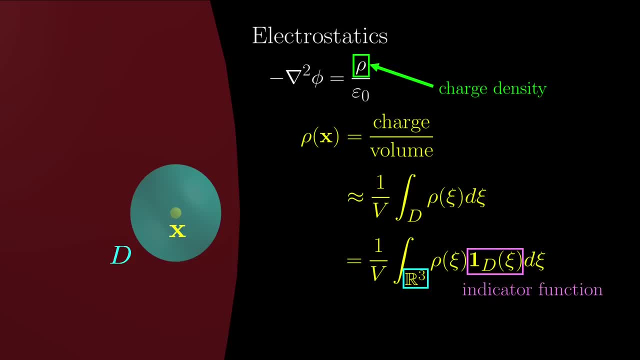 case indicating whether you are in region D or not, The function returns 1 if you are in region D and 0 if not. This trick works because the contribution of the integrand anywhere outside region D is 0.. The function returns 1 if you are in region D and 0 if not. This trick works because the contribution of the integrand anywhere outside region D is 0. 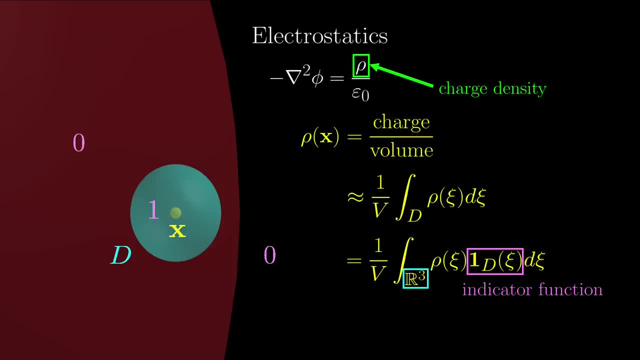 The function returns 1 if you are in region D and 0 if not. This trick works because the contribution of the integrand anywhere outside region D is 0. So you end up only considering inside region D anyway. Finally, because V does not depend on position, we can push it inside the integrand. 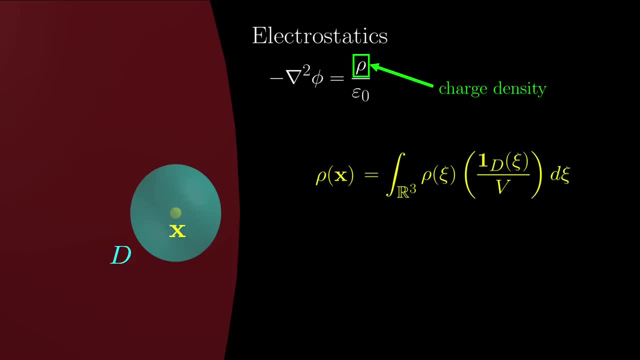 So now we have this expression of the charge density function. well, technically an approximation, but equal if the volume shrinks to 0. The good thing is that the only thing changing is this white boxed expression. This function takes the time to the infamous direct delta function when the volume shrinks to 0. 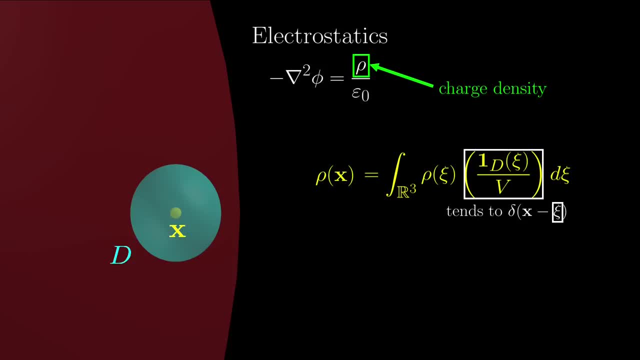 This depends on the position C, because the original functions before the limiting process depend on C, but also depends on x, because the region shrinks towards the point x. Anyway, now we finally get this expression involving the direct delta function. This might not look weird at first, but it is not. 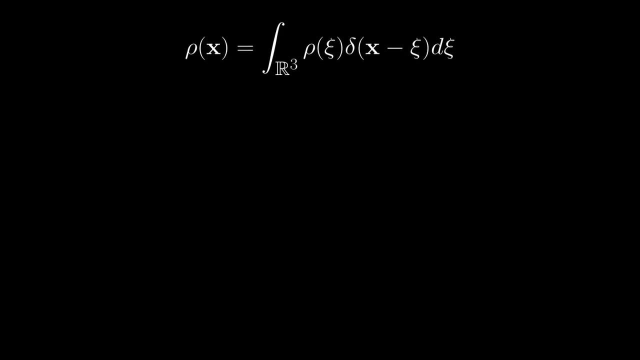 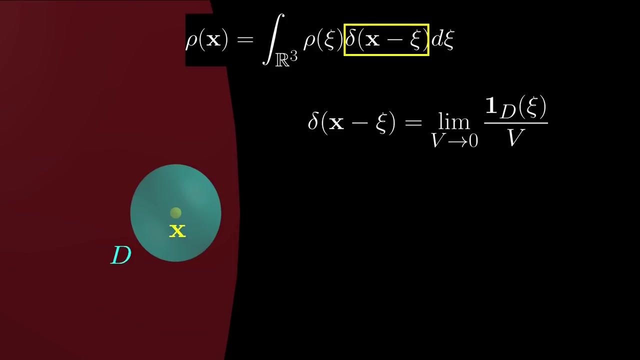 But as we explore a little bit more about the delta function, it will be weirder, But then we are going to see why this is not that weird. Let's go back to the measurement of charge density. As said just now, the delta function is the limit of this family of functions when the volume V tends to 0.. 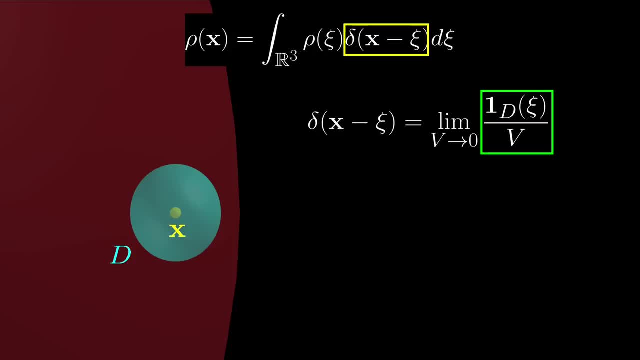 These functions are functions of position C. If C is not x itself, then the value of the function might initially be 0.. So if C is not x itself, then the value of the function might initially be 0.. So what if C is x? So if the rate of C is 0, and the delta function is actually 0,? men is tomorrow. 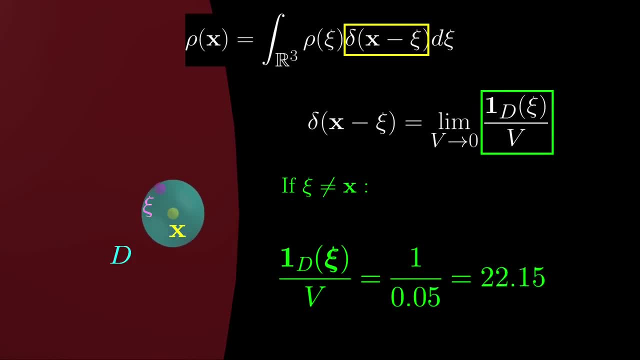 But what if C is x in the scan? It's possible that at that point the value of the function will also be lime. So this function is certainly going to be 0 at this point. So once again we have to calculate the Tourette's equation, in this case. 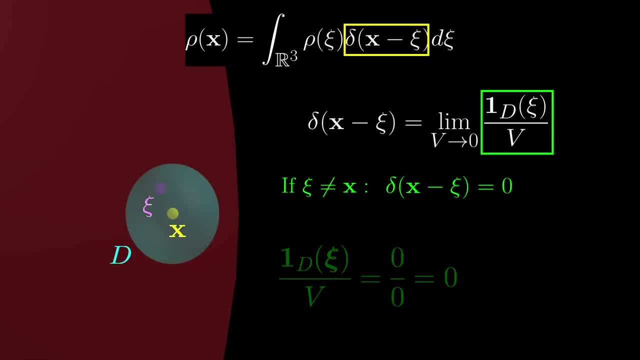 How about x? For our proof, x is 0, maybe 0+ 0, 0, 0.. the function would always return 1 throughout the limiting process, while the volume shrinks to 0, because, by definition, the region has to include the point x. So in the limit the 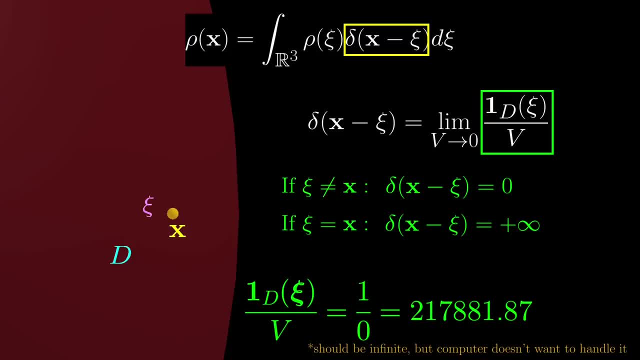 delta function shoots off to infinity. Simply looking at these two cases, isn't the delta function weird? Actually, this isn't even a function, because you can't define the value of a function to be infinity, at least not in this context. 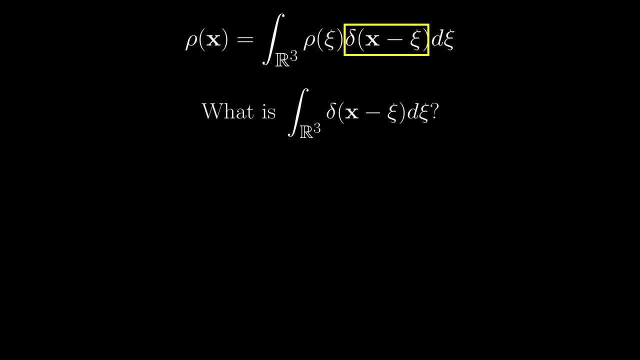 The weirdness continues. What if we try to integrate the delta function throughout space? We can use the formula at the top: substitute the charge density rho being 1 everywhere, then in particular the charge density at x is also 1.. In other words, integrating the 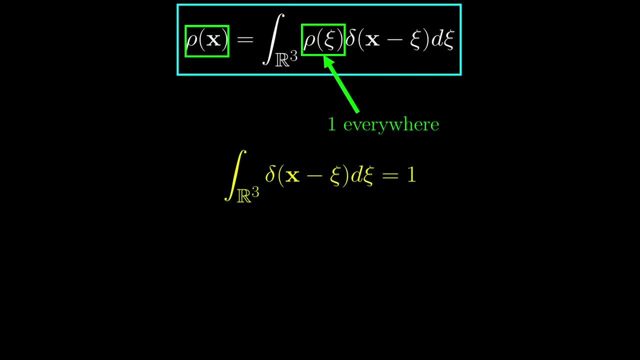 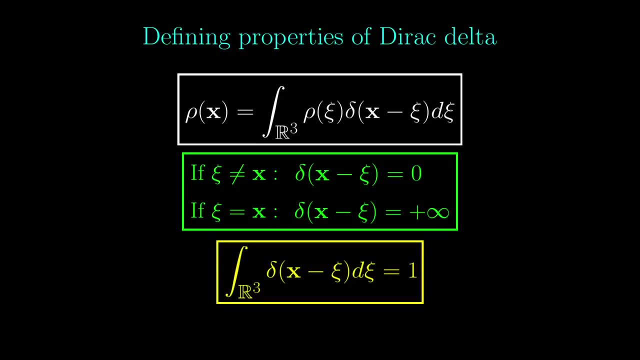 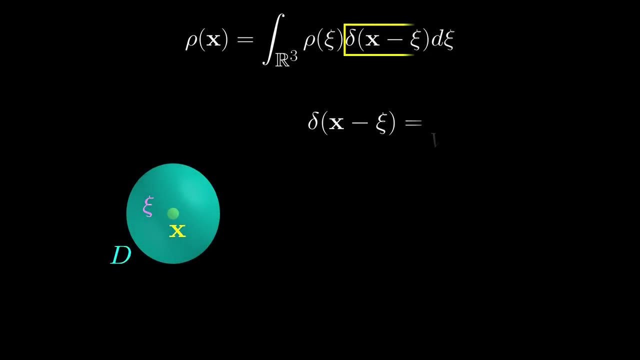 delta function throughout space gives you 1. These three things define the delta function And again, I know this can be weird, but I am going to convince you that it might be something you have seen before. Let's return to how we introduced direct delta in the first place, These functions of c before. 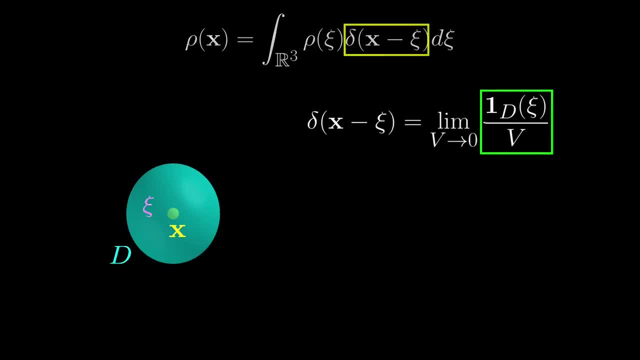 the limit are legitimate. What if we now consider this function to be our charge density distribution? Well, this means a uniform charge density within the region D, while the total charge is simply charge density, The charge density which is 1 over v multiplied by the volume v, which turns out to be constantly. 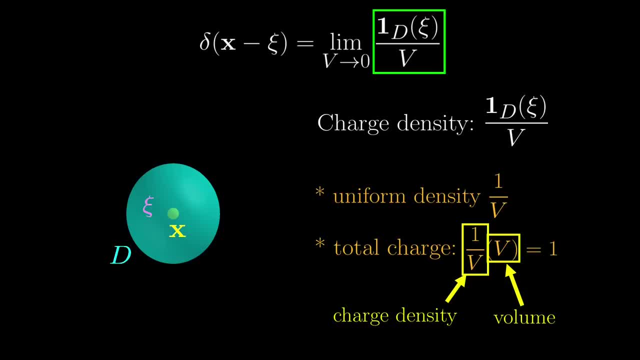 1, regardless of what the region is To obtain the delta function, we shrink the region down to nothing. So, viewed as a function of c, the delta function represents the charge density of a point, charge at x. This gives us some intuition on this expression In a very general. 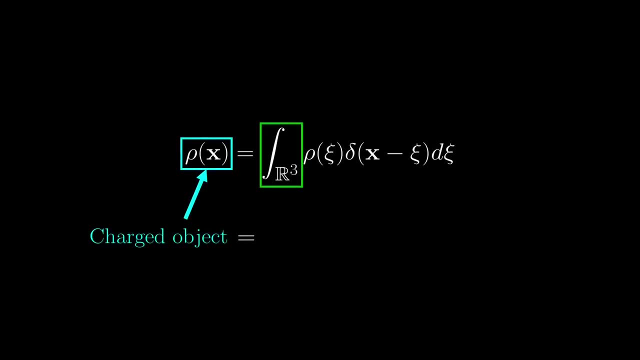 sense, a charged object is a function of a point charge at x. This gives us some intuition on this expression. In a very general sense, a charged object can be thought of as a continuous sum of point charges and the charge of each point. 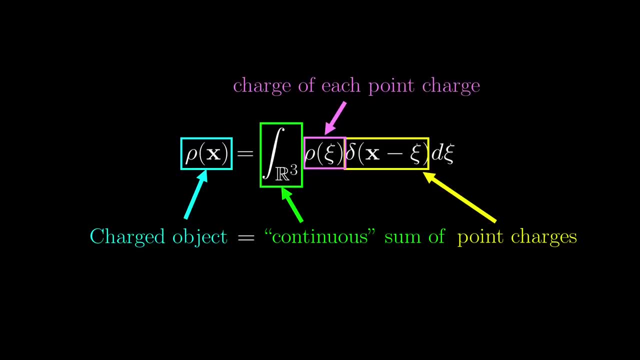 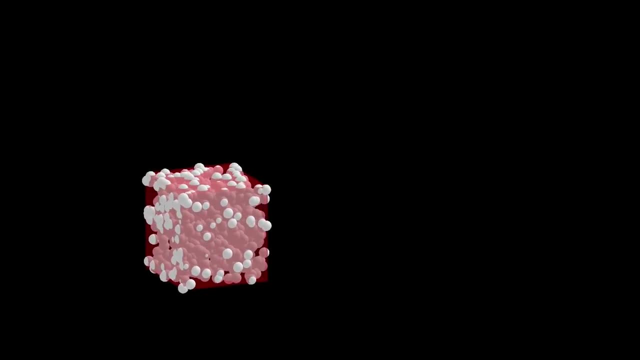 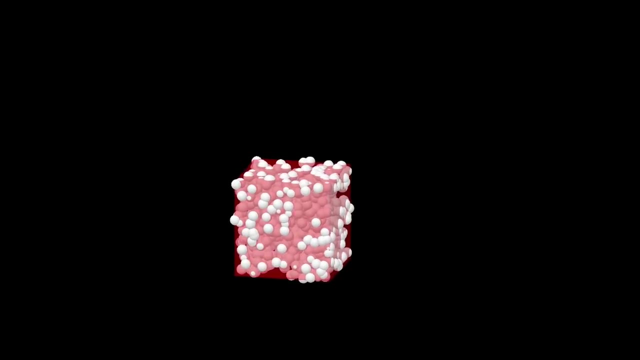 charge is governed by the charge density rho. This is a more mathematical expression of a pretty obvious concept, because nowadays we have the image that all objects are made of particles, in this case point charges. However, this is only a useful mental image. By no means is this an accurate depiction. 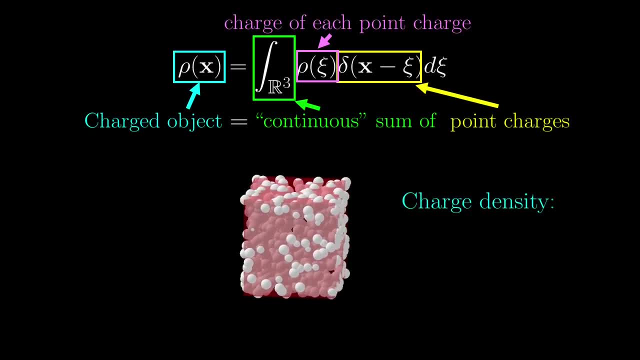 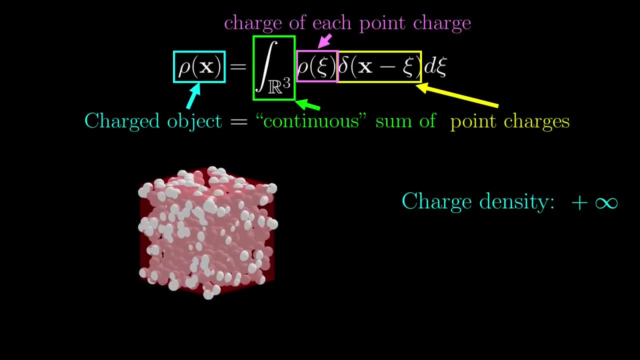 of a charge density distribution. Remember, this is just a reusable example and it is not necessary to refer to a single distribution. Otherwise the charge density at every point is infinite because there is a point charge there Instead. think of the reality as some blurred version of this. 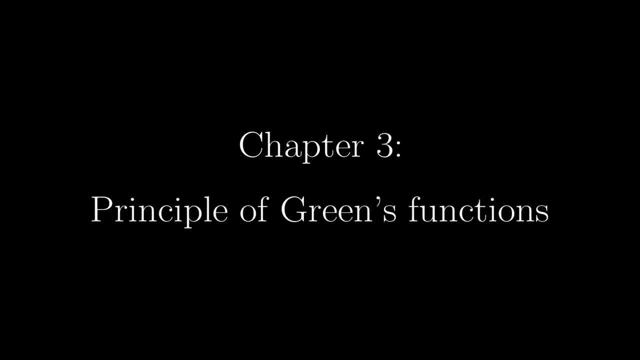 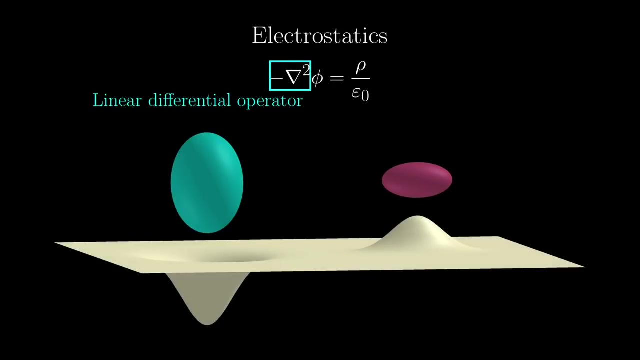 Let's return to the problem at hand. Given the charge density distribution function, we want to find the electric potential generated, and the method of Green's functions exploits the linearity of the operator. Remember that the operator being linear means that if we want to find the potential generated by two objects, we can find the electric potential. 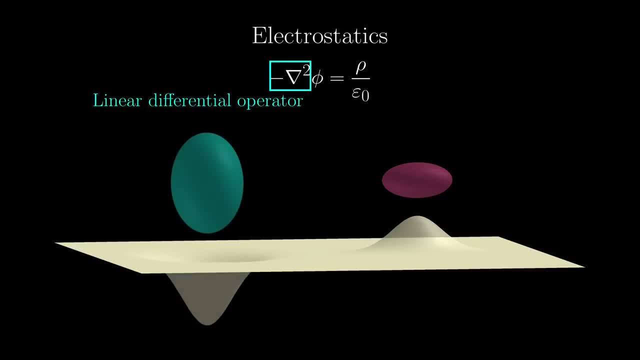 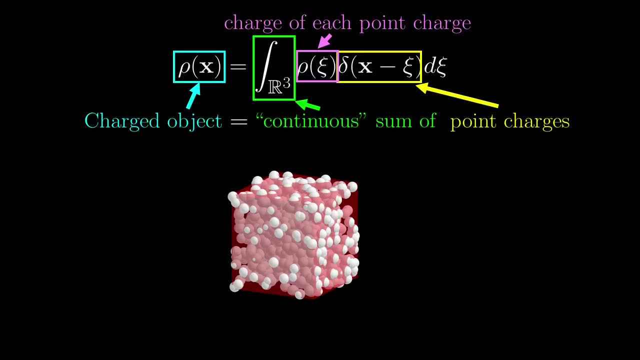 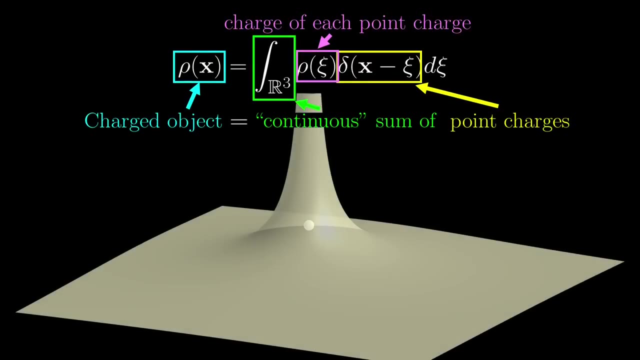 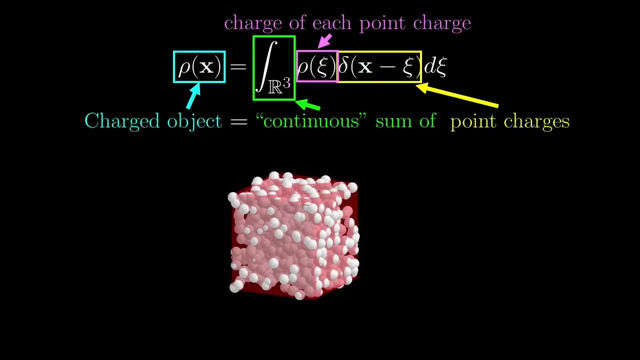 generated by each object first, Then simply add them all up. Now, given the previous interpretation of any charge density being a weighted continuous sum of point charges, we can first consider a point charge and find the potential generated, do the same for any other point in the charged object. then, from being a continuous sum of the point charges, 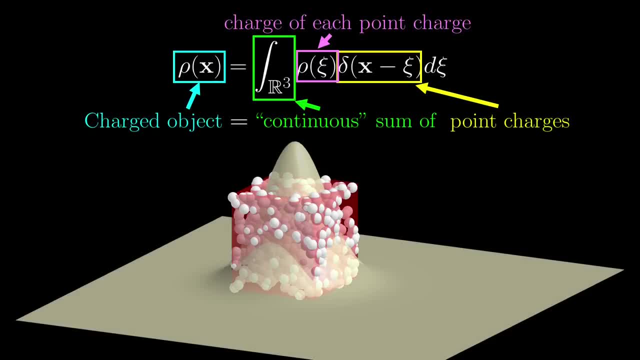 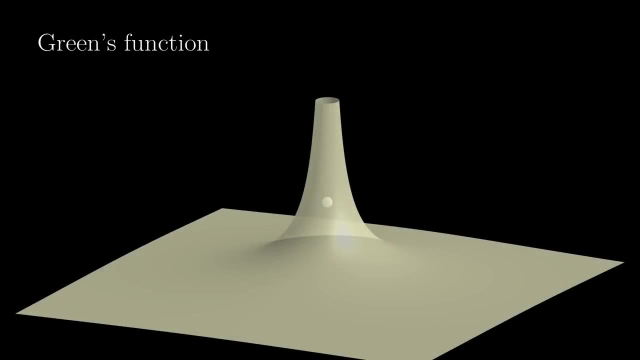 the electric potential can also be continuously summed. That is the overall idea of solving with Green's functions. Let's rephrase this a bit more precisely: The potential generated by a point charge in this context is the rescaled Green's function. The Green's function depends. 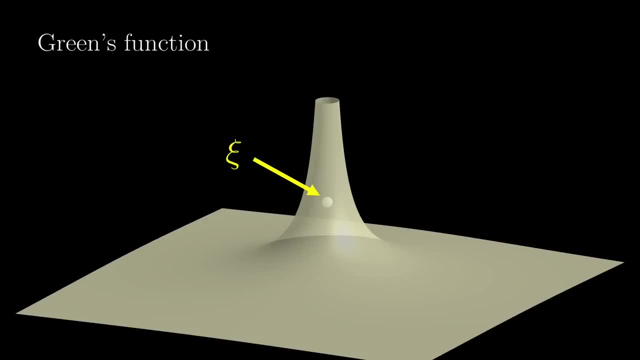 on both the location of that point, charge c, and the position where you find that potential x. So we denote the function as g, with two independent variables, x and c, while technically a rescaled one by epsilon naught, as I will explain shortly, The Green's function can be thought of. 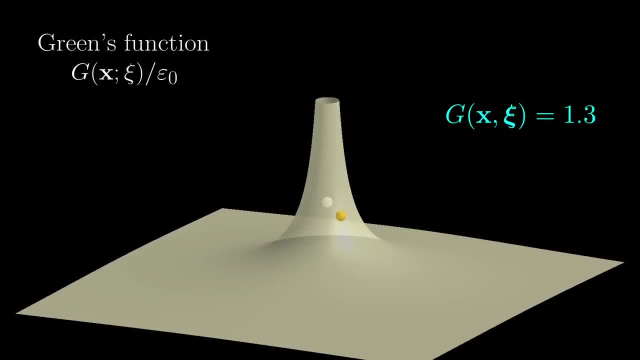 as a series of functions of x And which function to consider depends on c, And we want a continuous sum of these different functions. A continuous sum is more precisely an integral with a weight, the charge density. So the potential function should also undergo the same summing procedure, which means that we replace 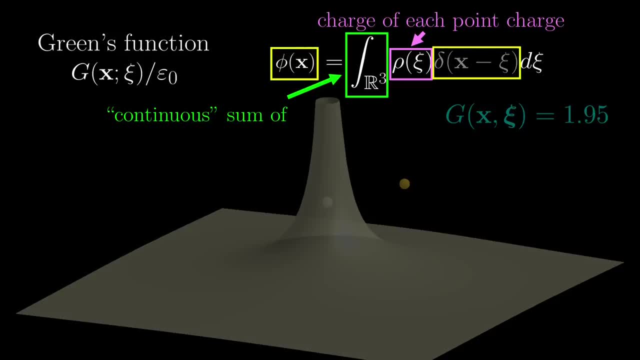 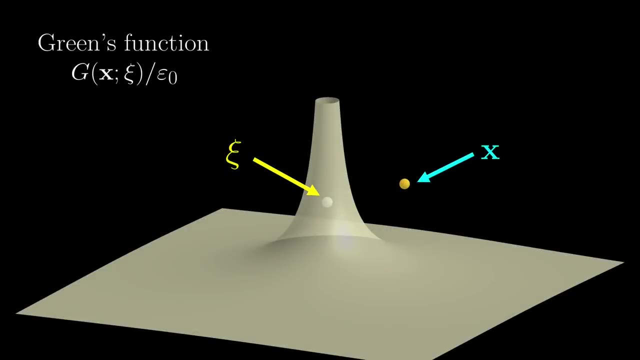 the delta function with Green's function, Then now the potential is a weighted continuous sum of the Green's functions. But why do we have to rescale the Green's functions? It all boils down to how we normally define Green's functions. Recall the related equation When we consider the potential for a point charge. 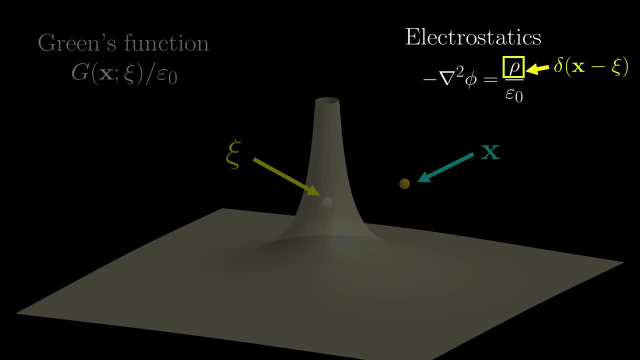 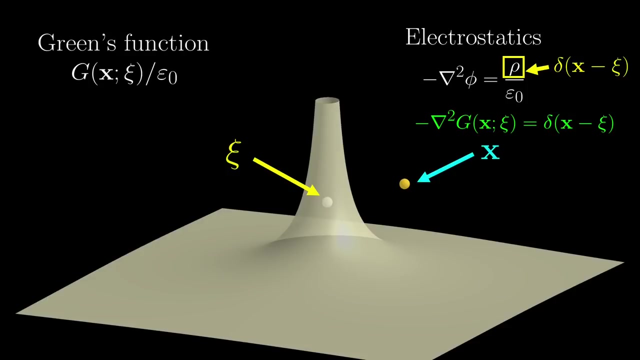 we essentially substitute rho to be a delta function, so the right-hand side has an epsilon naught. However, we normally define the Green's function to be only having the delta function on the right, so we have a factor of epsilon naught to deal with. That brings us to a sort of summary. 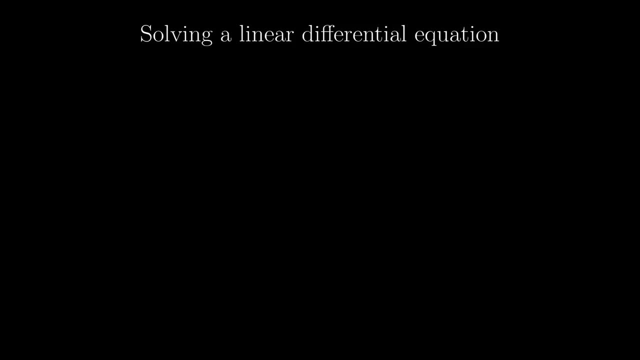 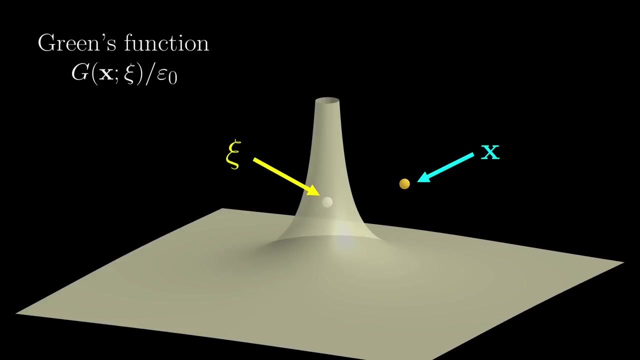 and a more algebraic way of looking at all these. The equation we are interested in looks like this and, most importantly, L is linear. First off, we find the Green's function, which is the equivalent of finding the electric potential generated by a point charge. 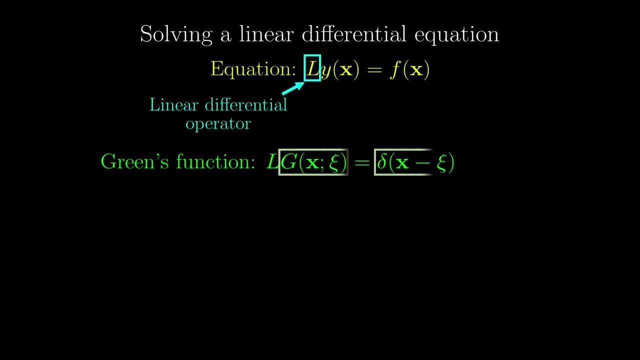 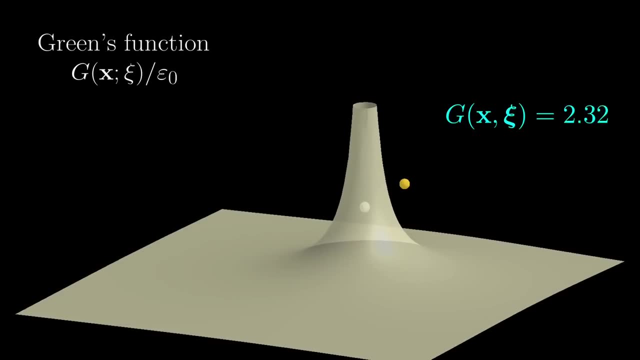 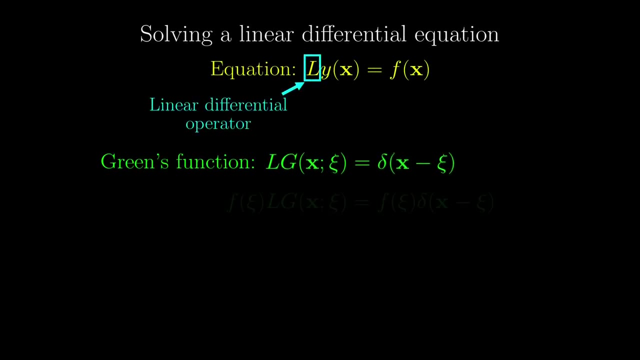 The Green's function and the delta function should be viewed as just different functions of x, which means something like this: different potentials generated by point charges in different positions. After finding the Green's function, we multiply both sides by f. Now this f. 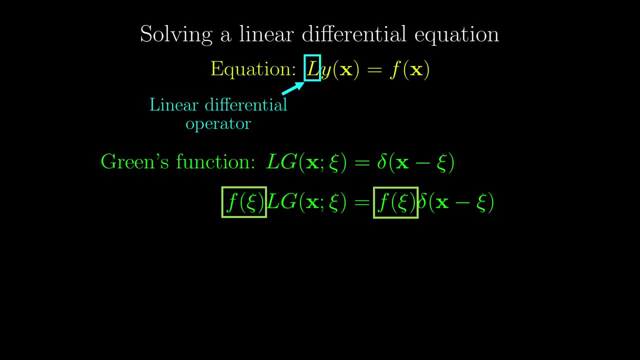 does not depend on x, and so it is a constant in L's perspective. In other words, we can swap the L and f- This is true for all c- and so we do the so-called continuous sum of the previous relation. The right side is precisely the continuous sum of point charges. 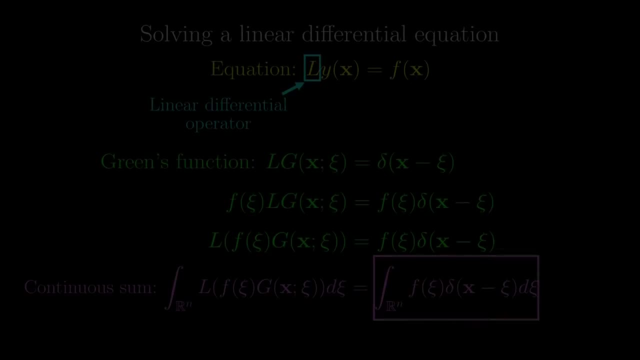 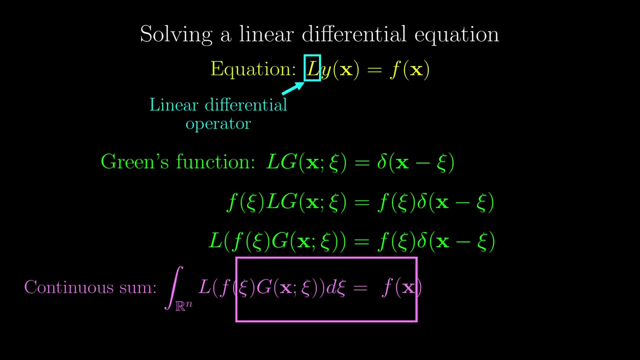 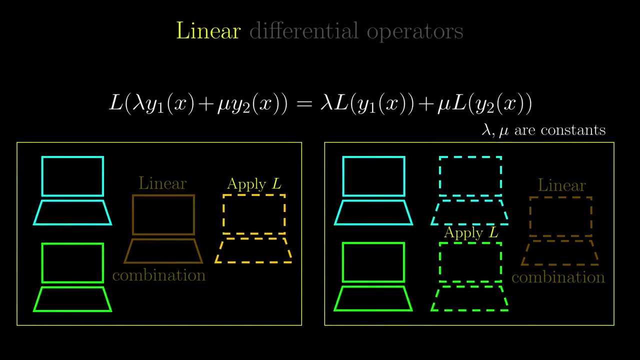 thing I've said in the previous chapter. so the box on the right hand side is precisely f. However, the left side is just slightly trickier. Remember that L being linear means that the steps of applying the operator L and linear combination can be swapped without affecting the final result. 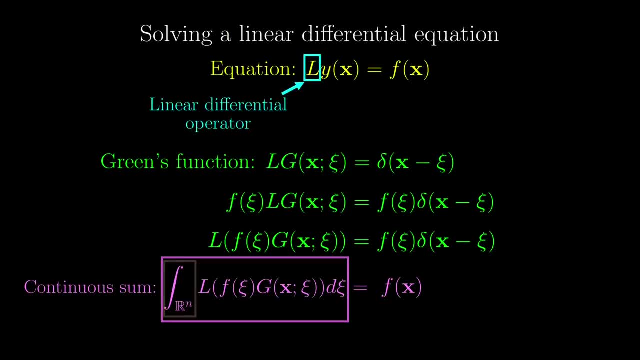 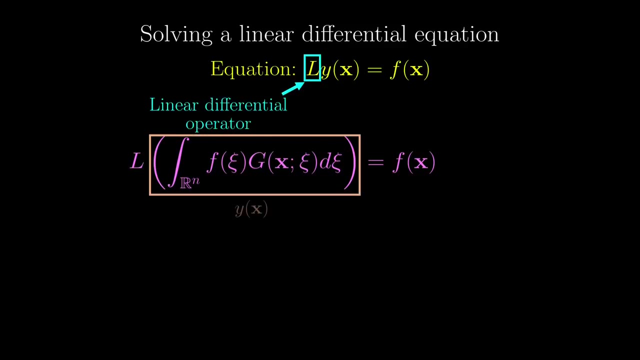 Here on the left hand side. since the integral can be thought of as an infinite linear combination, it can also swap with L, and so we just swap them. Now compare with the equation we want to solve. If we call the thing inside the bracket to be y, 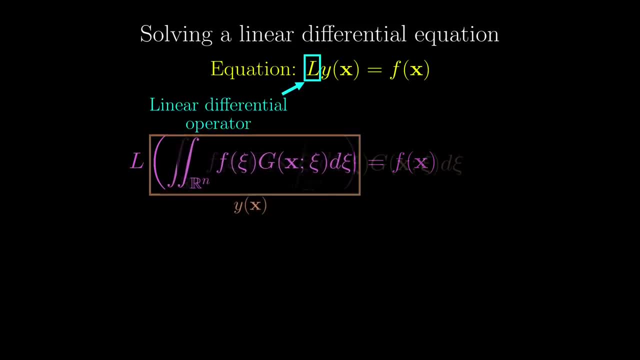 then this precisely solves the equation. Isn't that genius. If we know the Green's function g, we can just plug f and g into this to find the solution. There are a few quite important questions that we will briefly go over in the remainder of this. 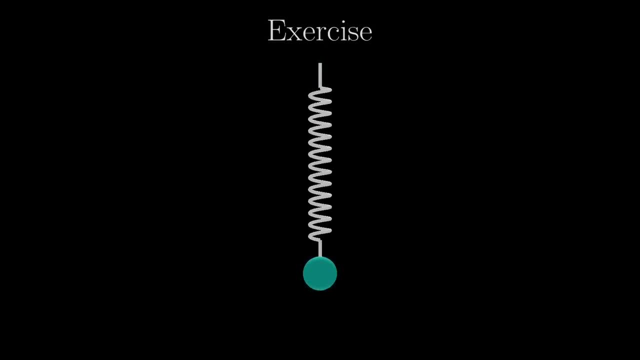 video. but before that I think it is a good exercise to think through another example from physics with the same framework in this video. In this example, x refers to the extension from an equilibrium position and f refers to the applied force at time. t As an exercise, and 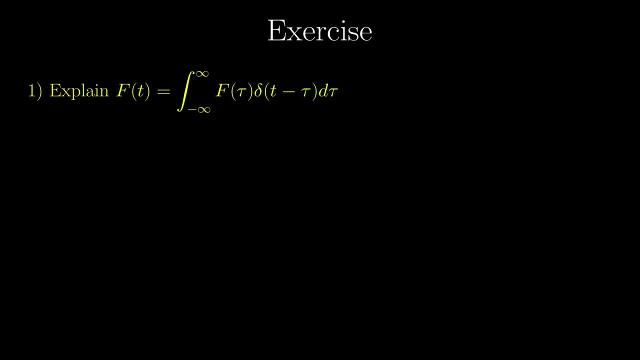 honestly, a kind of summary. first explain why the applied force can be written this way, directly from the fact that force is the rate of change of momentum. Then come up with an intuition of the delta function, which should be some analogue of point charge. Then reinterpret the formula as some sort of continuous sum. and what the 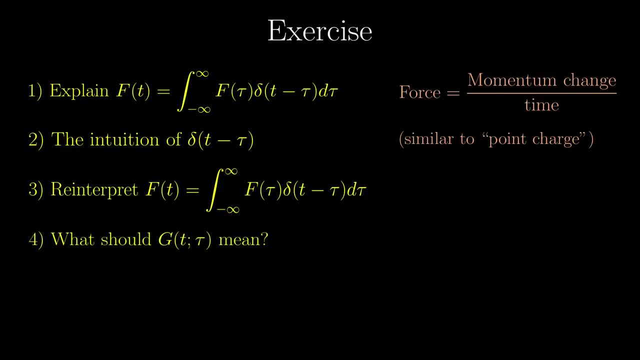 Green's function in this case means. Finally, what does linearity of the operator mean in this context and thus interpret the final solution involving Green's function? Remember, the context is an oscillator with an applied force. Pretty much the same procedure in the. 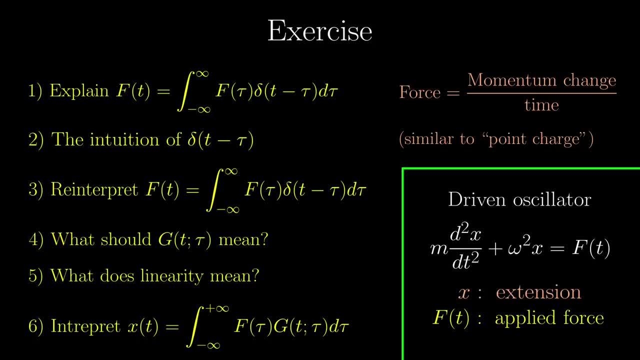 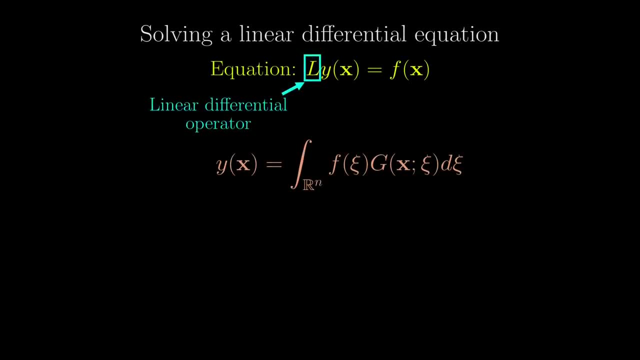 video, just with a different context and equation. To solve the differential equation by applying the formula in this video, you first have to find that Green's function. But how? Here's a very brief overview. Remember that by definition, the Green's function satisfies. 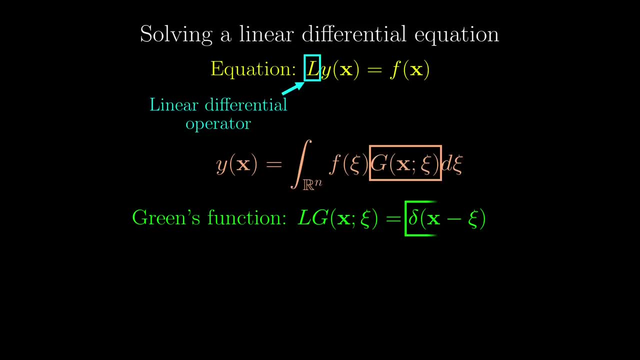 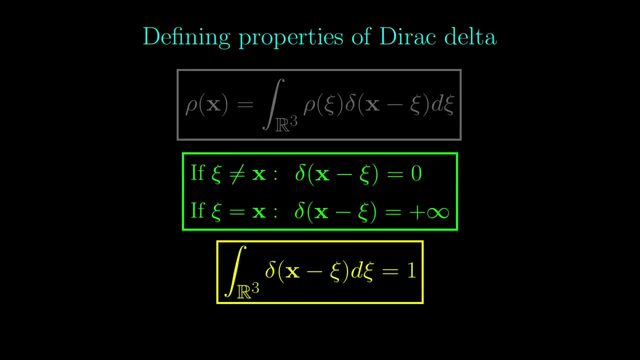 this equation and the method hinges on the properties of the delta function. The delta function has these defining properties, in particular these two: It is 0 almost everywhere, and integrating throughout space gives 1.. Well, no, precisely because it is 0 almost. 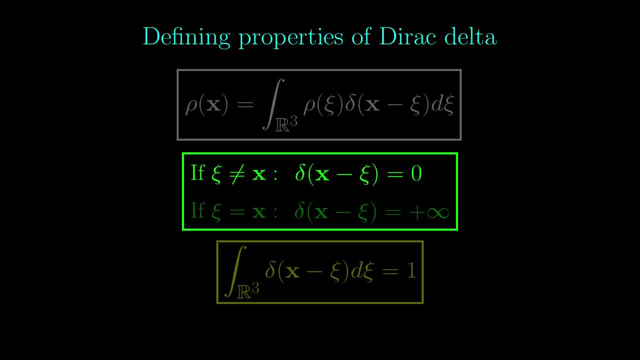 everywhere. the integrand gives 0 contribution almost everywhere, almost everywhere as well. so we don't need to integrate throughout space, just the small region D, as long as it contains the point x. and then we simply apply these two properties to the equation for Green's function, ie solving the equation where the right hand 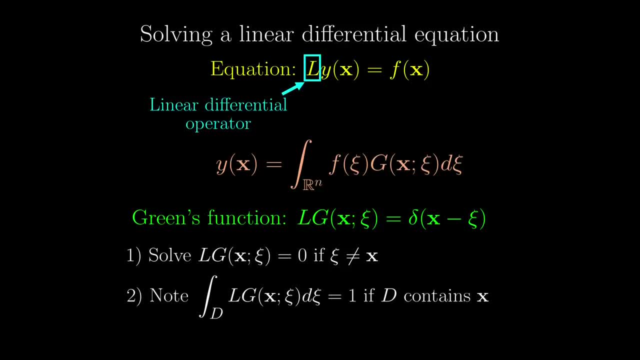 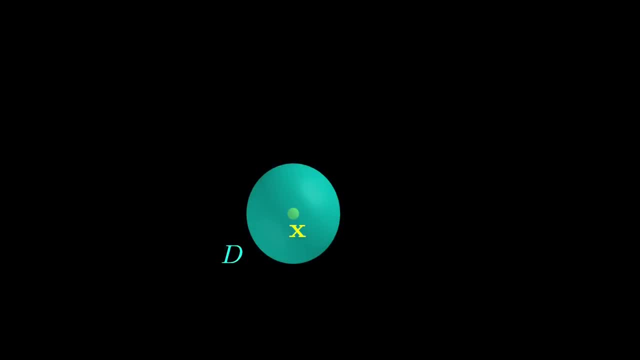 side is 0 almost everywhere, and integrating it in any region D that contains x would give 1.. The region D is cleverly chosen, in this case a sphere, to make life easier, and sometimes you might even want to shrink the region D as small as possible. 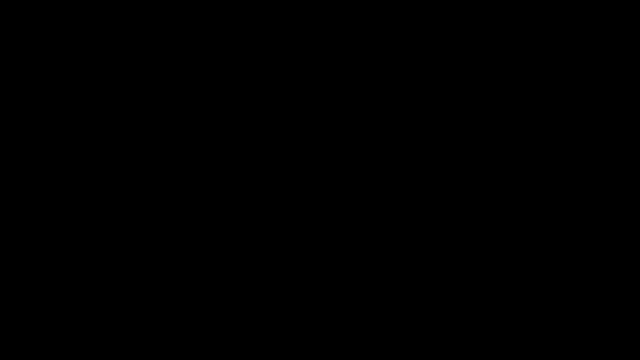 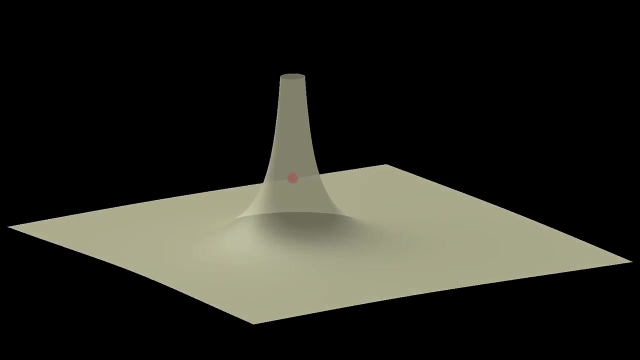 Another trick to simplify would be to consider symmetry, like in this case, a point charge. However you try to rotate, you see the same physical setup, ie the setup has a rotational symmetry, and so we expect the potential to also inherit the same kind of rotational symmetry. 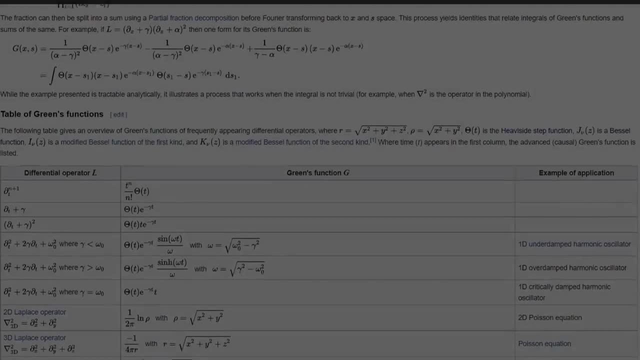 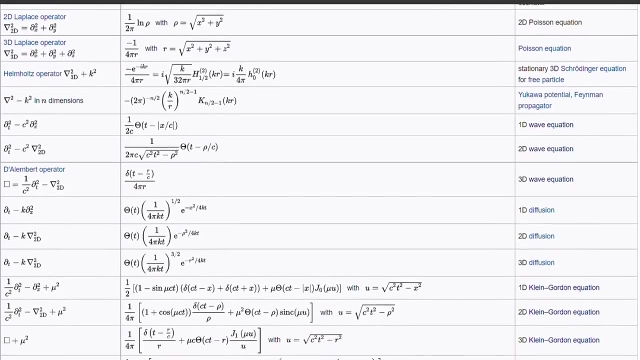 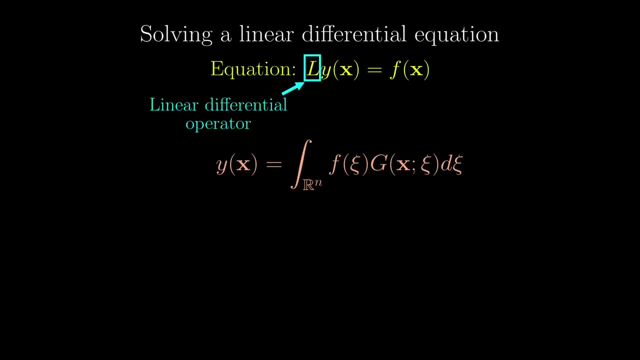 But actually, in practice, you don't even need to find the Green's function yourself. this Wikipedia page already lists the Green's functions for most common linear differential operators. Looks like everything's good now right In order to solve a differential equation, as long as we have the Green's function. 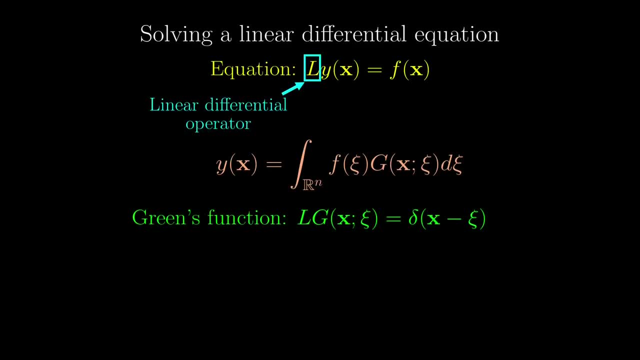 we are ready to go, and the Green's functions can be found pretty easily online, But there is usually something much, much messier to deal with. So let's get started. 1. Let's reuse the point charge example to illustrate further problems with finding. 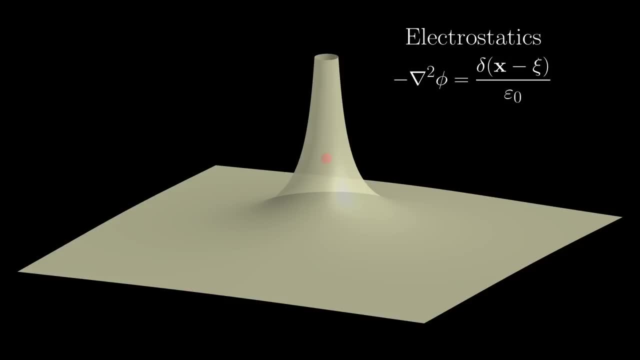 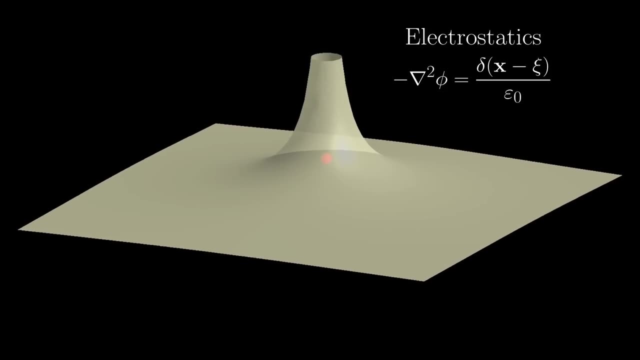 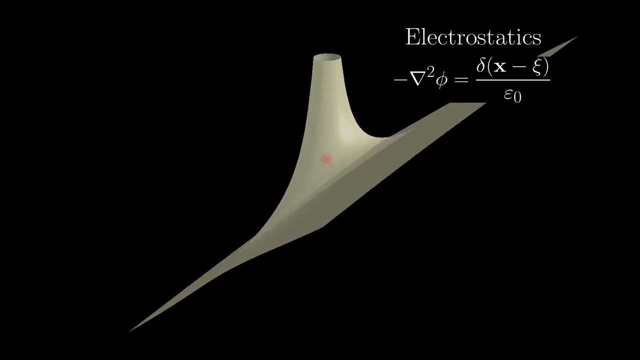 the Green's function From a purely solving equation perspective. this is not the only solution. For instance, adding a constant would actually still solve the equation. Well, you know what? There are even crazier changes that can make the equation still satisfied, but we only. 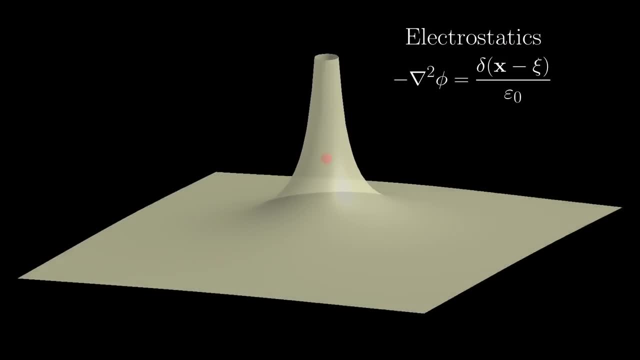 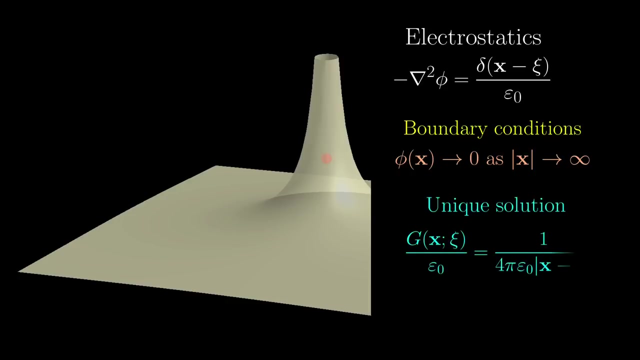 want one, So we impose some extra restrictions like boundary conditions. In this case, The implicit boundary condition is that the potential dies when it is very far away from the point charge and it turns out there is only one solution after we impose this extra. 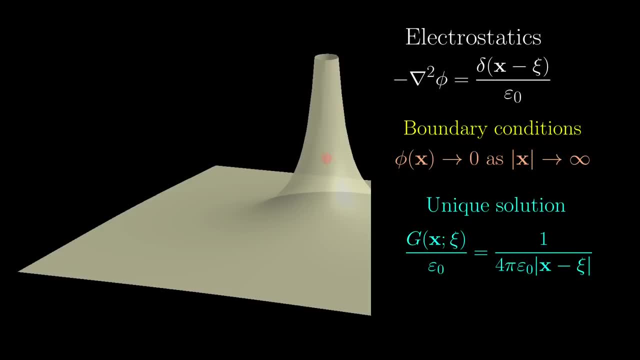 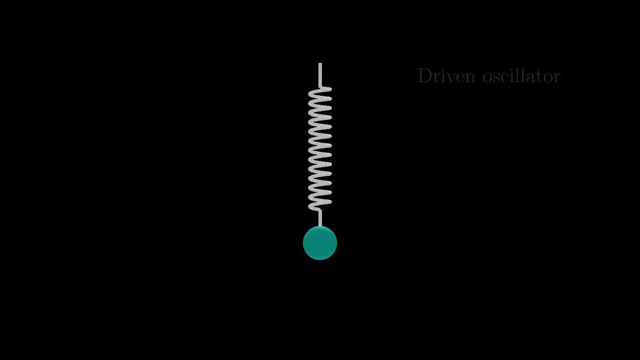 restriction, But starting with different boundary conditions, we would obtain different Green's functions For physical systems where we are interested in time evolution. we also need to impose some extra restrictions so that there is only one solution, In this case initial conditions, like the initial position and the initial velocity. 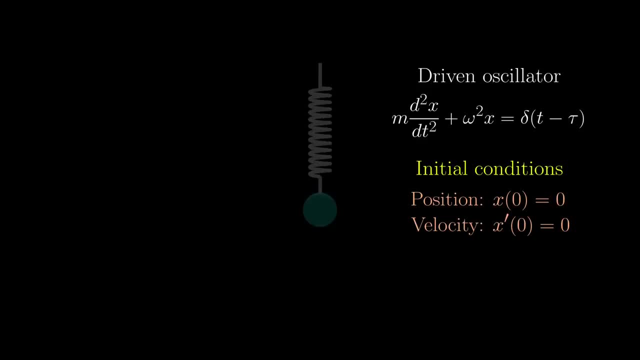 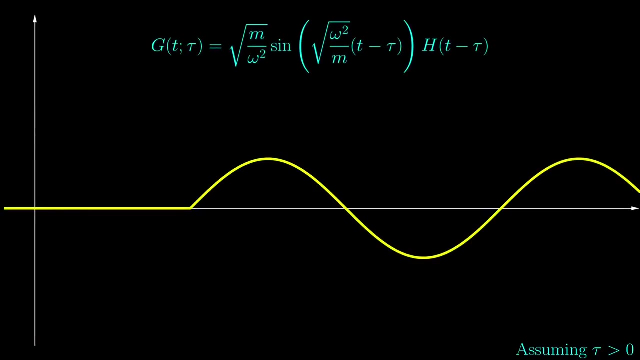 And the usual convention is that they are both 0.. Again, after imposing these initial conditions, we finally get a unique solution. This solution looks a little bit intimidating, but really it's just a delayed and rescaled sine wave, starting at time tau. 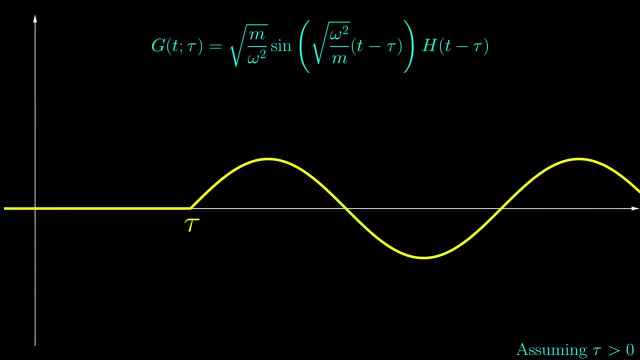 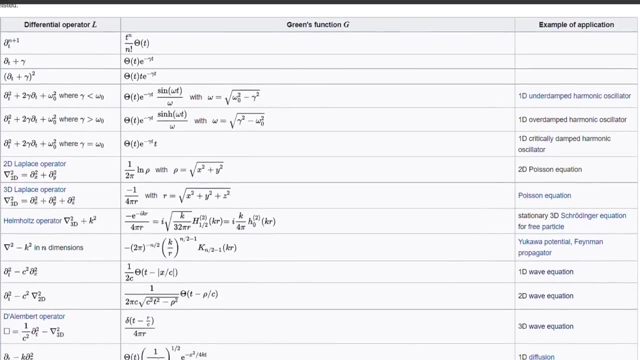 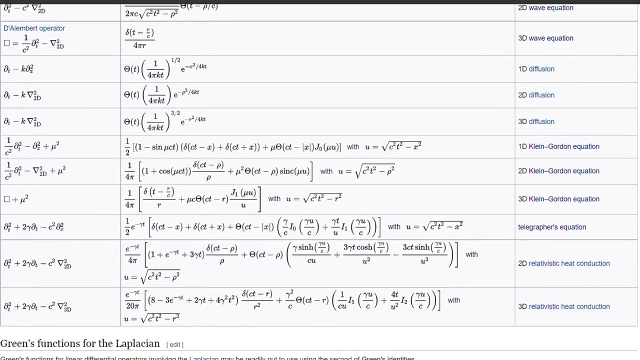 Again, different initial conditions would result in different Green's functions 2.. So when you look up the table for Green's functions online, it is important to see what kind of boundary or initial conditions they are assuming, explicitly or implicitly. In these two cases, the extra restrictions are quite nice, being 0 on the infinite boundary. 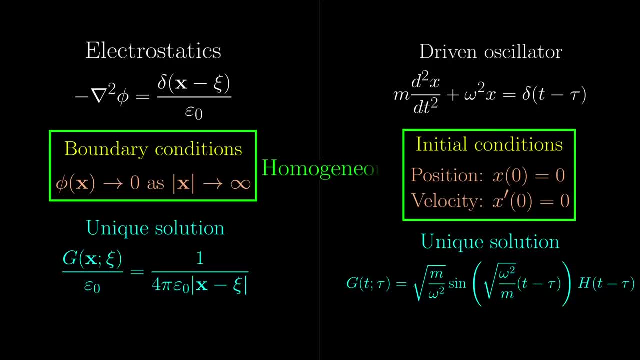 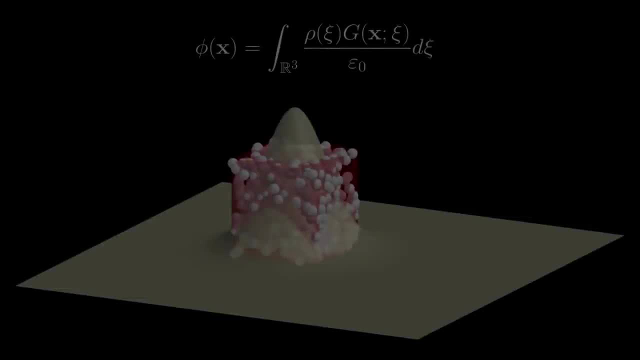 or 0. initially, These conditions are called homogeneous where the 0 function satisfies. As we know, the ultimate solution is a way to solve the problem. So let's look up the table for Green's functions online. It is important to see what kind of boundary or initial conditions they are assuming explicitly. 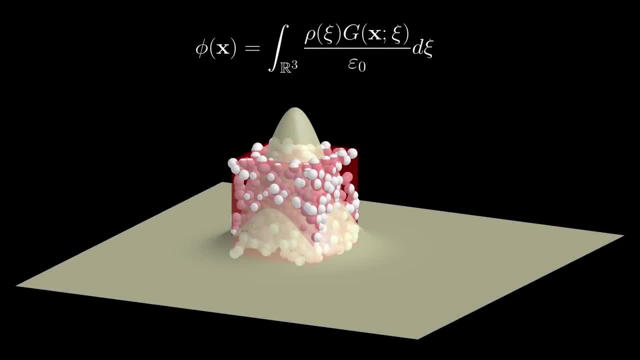 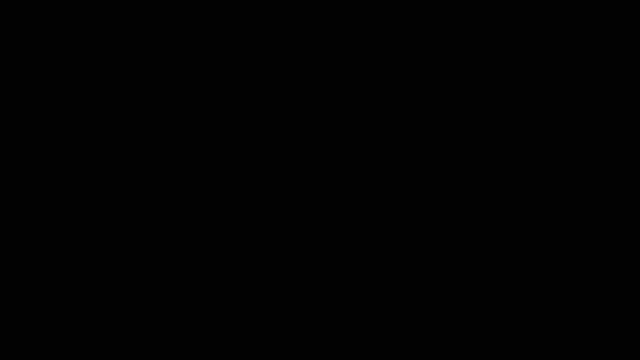 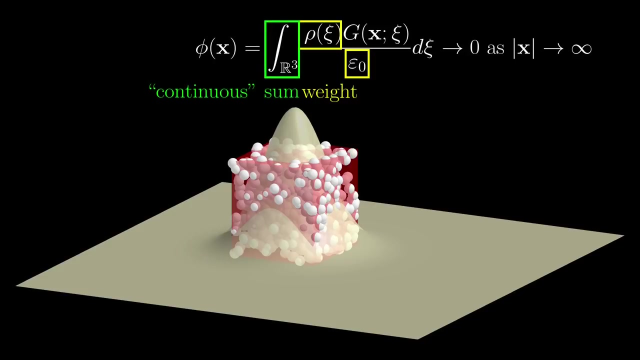 or implicitly. If we insist that all the individual Green's functions obey this boundary condition as long as the weight is sufficiently confined, adding up these Green's functions would also obey the same boundary condition, simply because adding 0 a bunch of times still gives 0.. 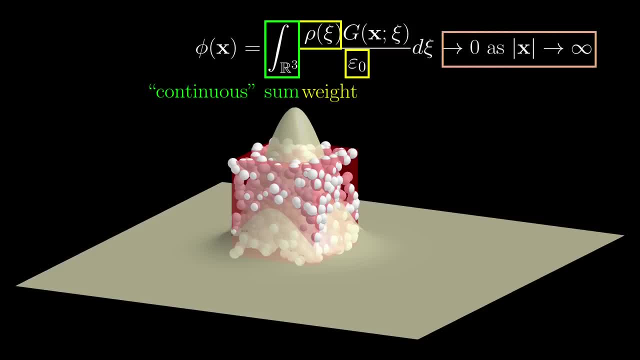 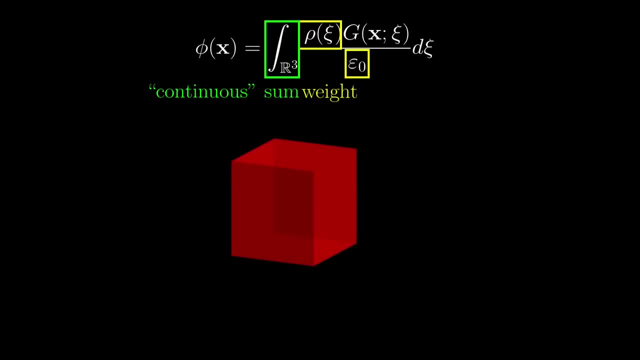 This is something good if we wanted this boundary condition in the first place. If, however, we wanted to add a number to the boundary condition, then adding 0 would still give 0.. If we want a different, more complicated, inhomogeneous boundary condition like the: 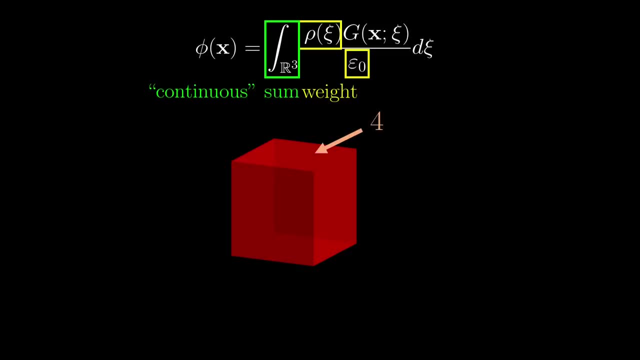 potential being 4 on a top face but all the other faces having potential 0,, then there isn't an easy way to directly apply the Green's functions technique. If you have found a Green's function, ie the scaled potential for a point, charge for. 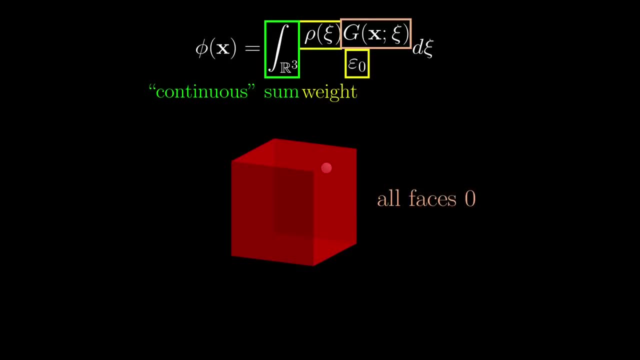 which the potential is 0 on the entire surface of the cube, then adding these potentials together would give 0.. If we want to add another number to the boundary condition, then adding 0 could be more complicated. so we can add 1 to the square root of 1 and add 1 to the square root of 3.. 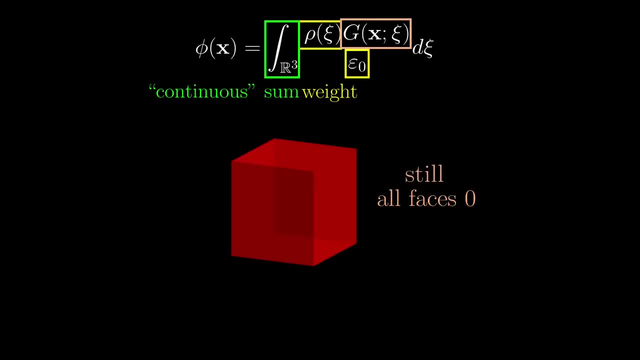 If we add another number to the square root of 3, the square root of 3 ends up adding the same potentials. Now we have filled out the entire boundary of the problem. If we want to make the case that the upper face is 0 instead of 4, these cases will. 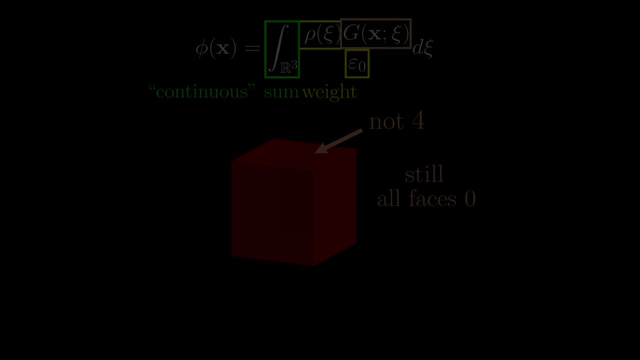 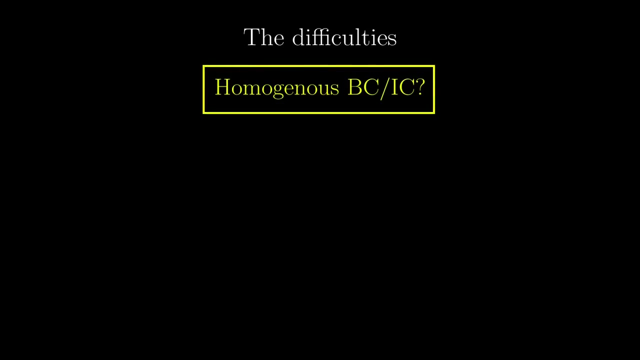 be much trickier to deal with. As a small summary of this chapter. basically, we need to first ask whether the problem has homogeneous boundary or initial conditions. If not, then the method of Green's functions can't directly help, but it might help in.